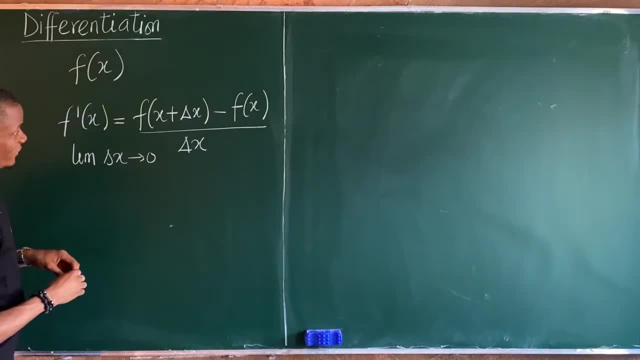 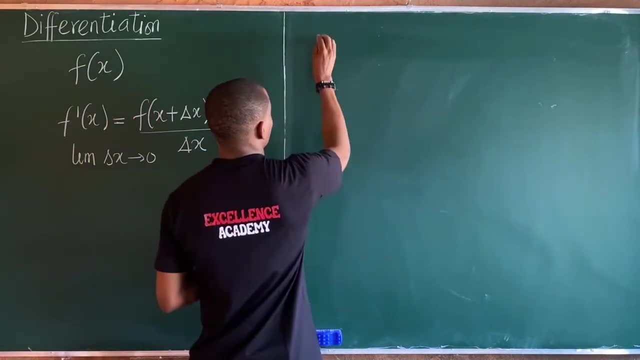 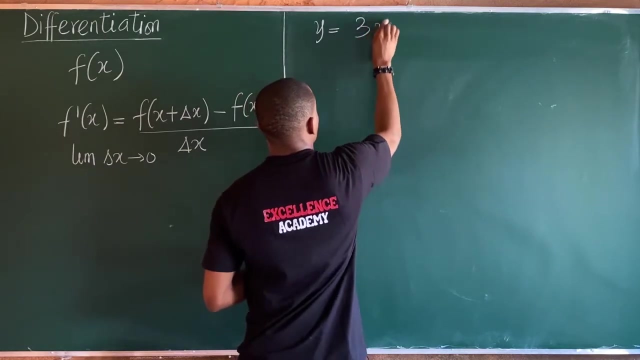 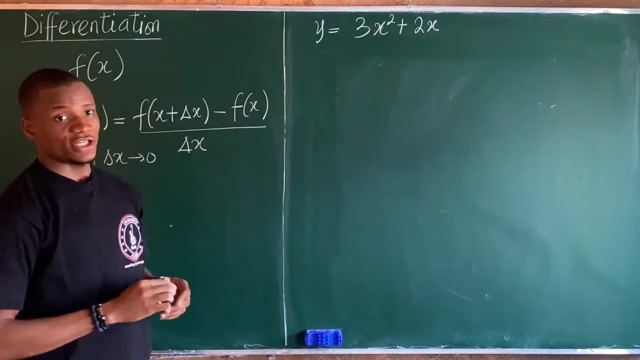 first principle formula of differentiation. I'll explain this using a very simple concept. Let's say I have y being equal to 3x squared plus let's say 2x, for instance. I'm asked to differentiate this using first principle. Do a guesswork From this. if I use general method, 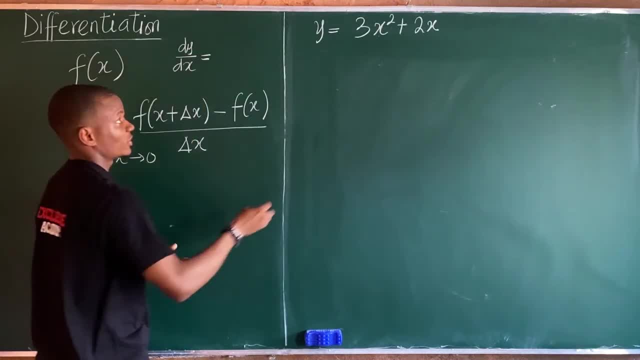 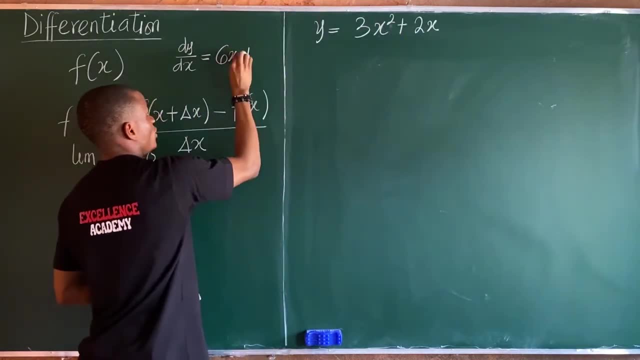 I'll have that. the y over the x from general method is this times this, that's 6x, into 2 minus 1, that's 2 plus. in this case it's just 2 and x standing alone. It becomes what there 2 by. 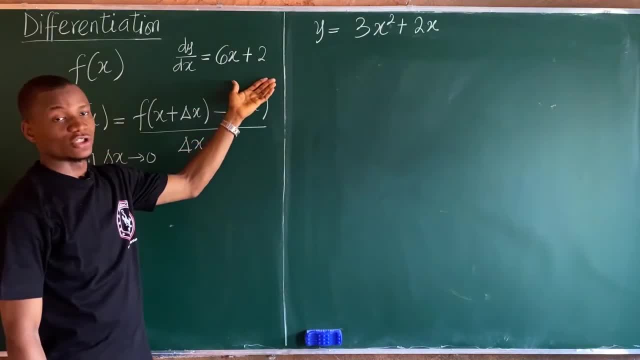 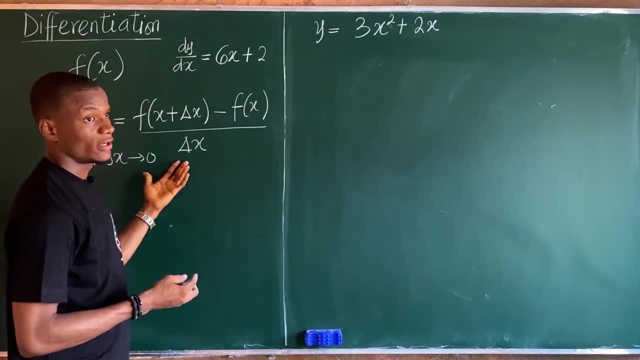 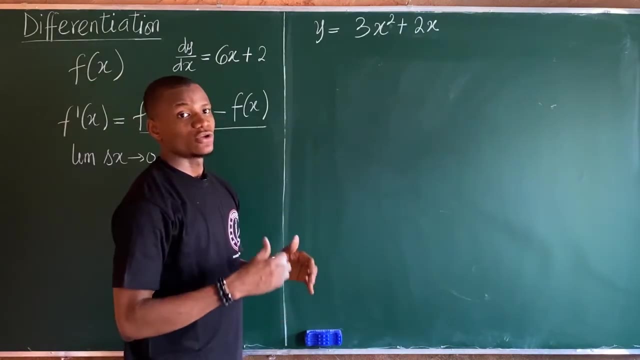 differentiation. I'll have this using general method. You could perhaps factorize here if you wish. But let's look at how to solve this using first principle formula. So it's just the same principle From here. we said: to y, add change in y. to x, add what there Change in x. So I'm having y. 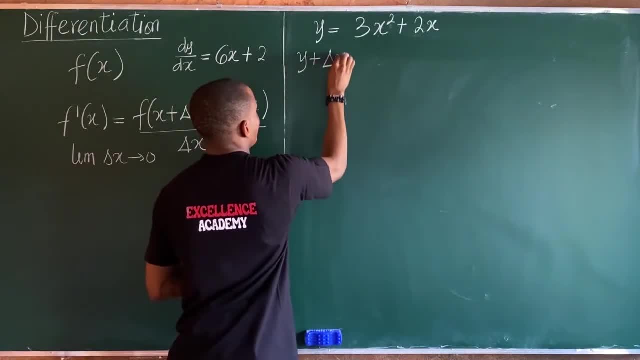 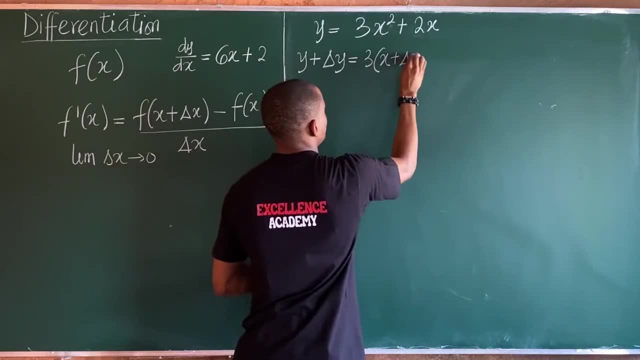 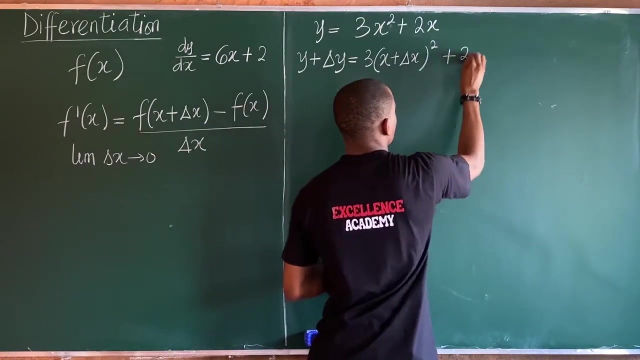 here becomes y, plus change in y is equal to it becomes 3. here I'm having x. squared becomes x, add what there Change in x. This man is squared, becomes squared here, plus next up I'm having 2 into. here is x. add what there Change in x. So I'm having y plus change in y is equal to 3. here I'm. 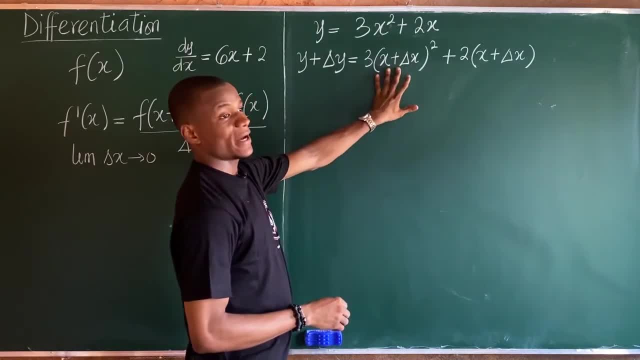 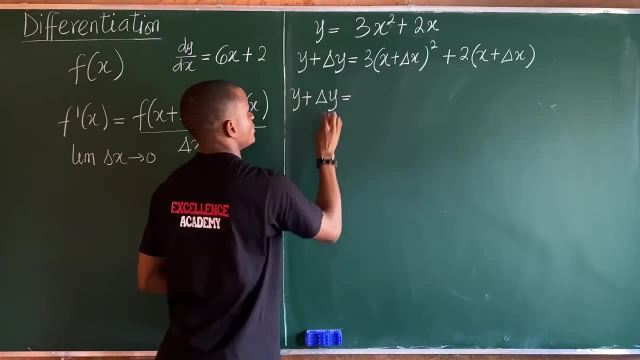 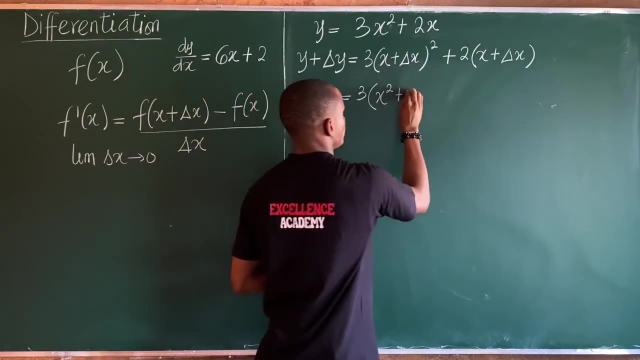 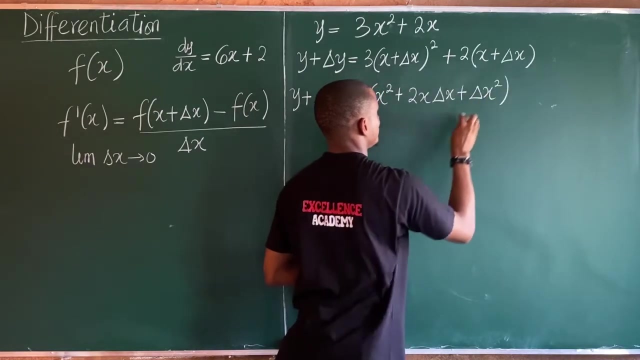 having x- So I'm having this Next up now I'll expand this and try to simplify. So this gives you y plus change in y is equal to 3- into. if I expand, this becomes what there- x squared plus 2x change in x plus change in x squared. That's for the expansion of this plus 2 into what there. 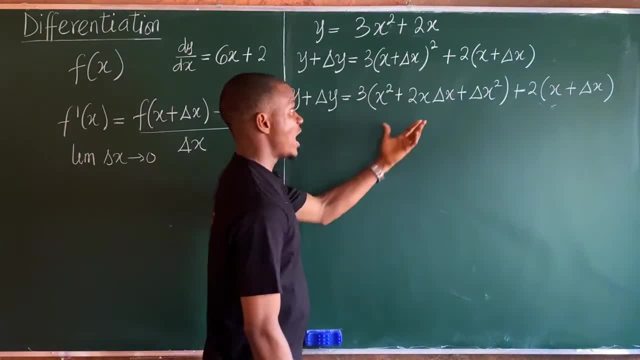 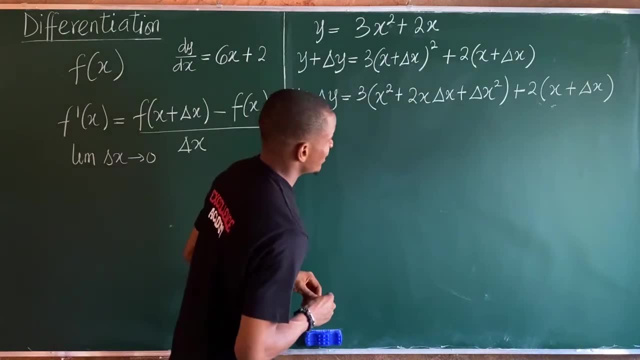 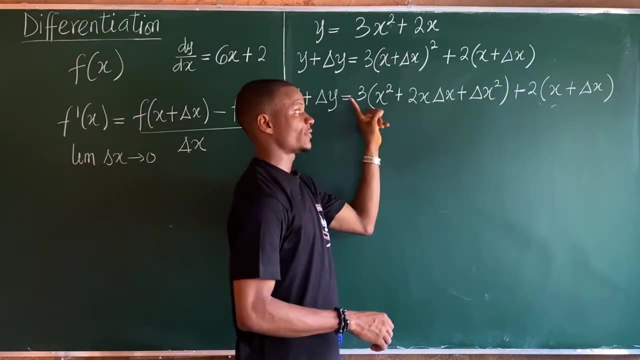 x, So I'm having this. I already explained this in the previous video, So you could go back to the previous video and see how I expanded this. All right, Next up now I'll have to multiply 2.. That means I'll expand this bracket. Multiply all of these by 3.. Multiply this by 2.. So I'll have that. 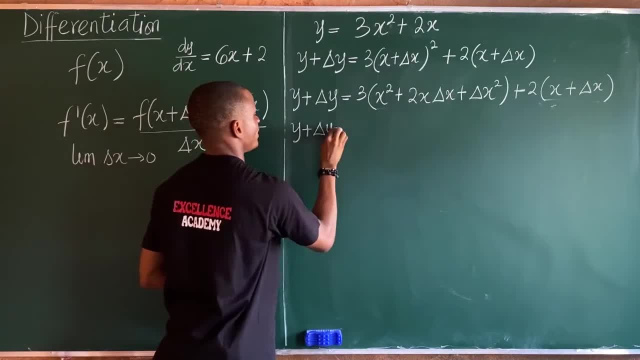 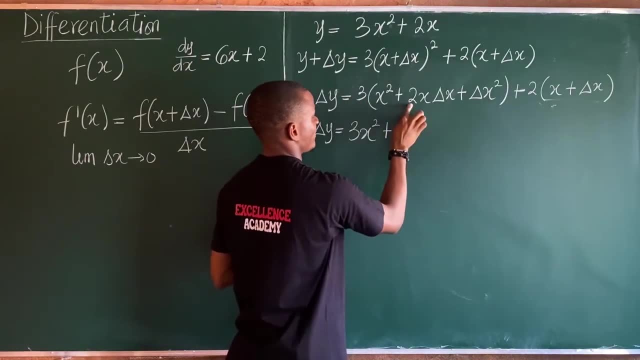 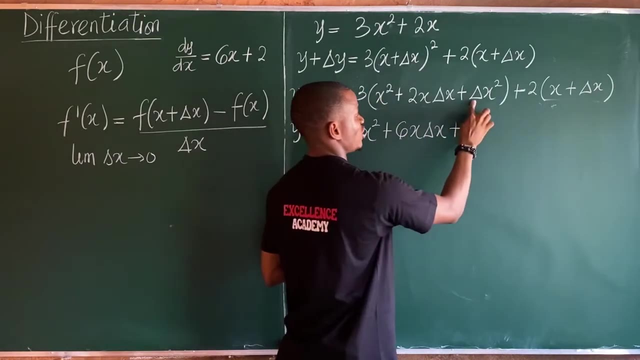 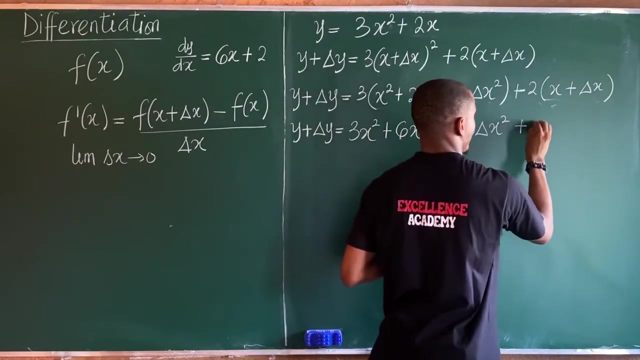 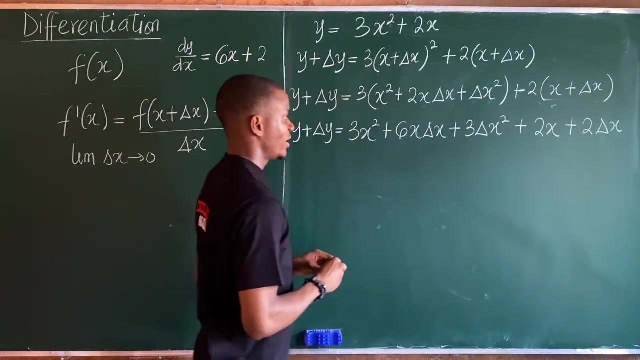 y plus change in y is equal to 3 times x squared, gives you 3x squared Plus 3 times 2 gives you 6.. I'm having x change in x plus 3 times change in x squared gives you 3 change in x squared plus 2 times x gives you 2x, plus 2 times change in x gives you 2 change in x. 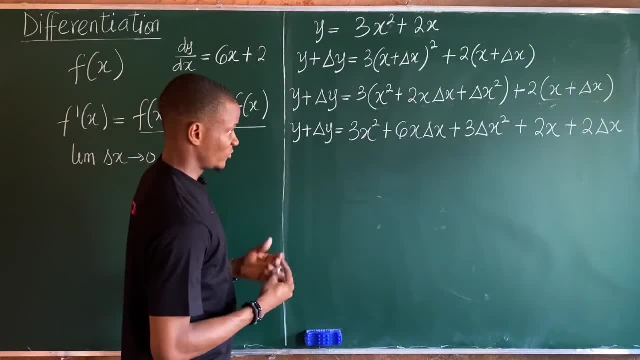 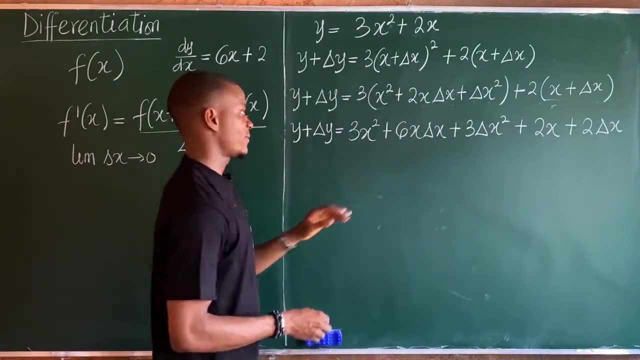 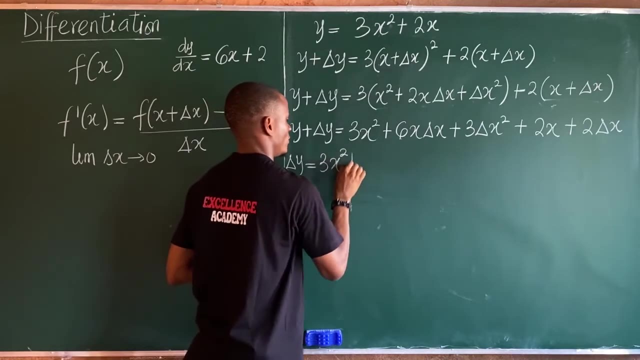 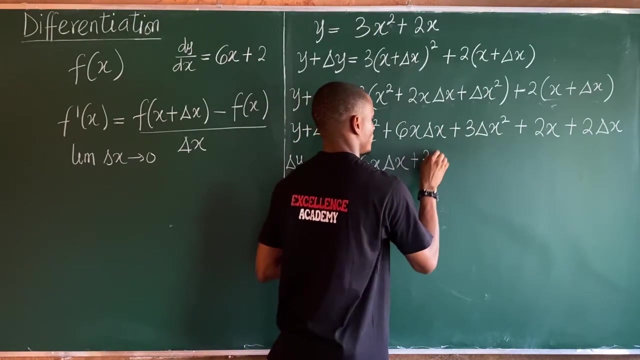 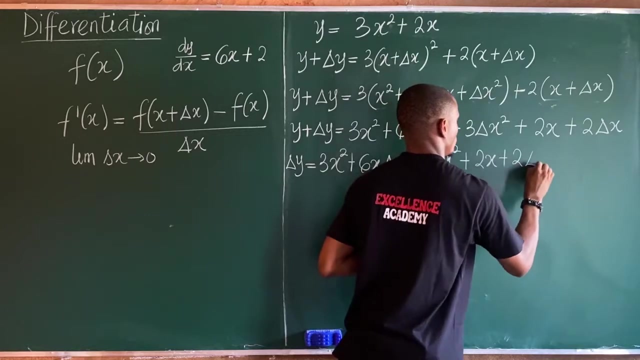 Next up. I'll look at this. Are there like terms? No, No, like terms. So next up, I'll move y over here, Move y over here. So I'm having that change in y is equal to 3x squared plus 6x change in x plus this 3 change in x squared plus. I'm having this as 2x plus 2 change in x. 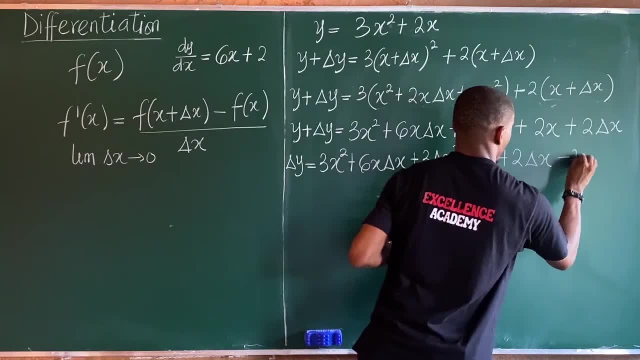 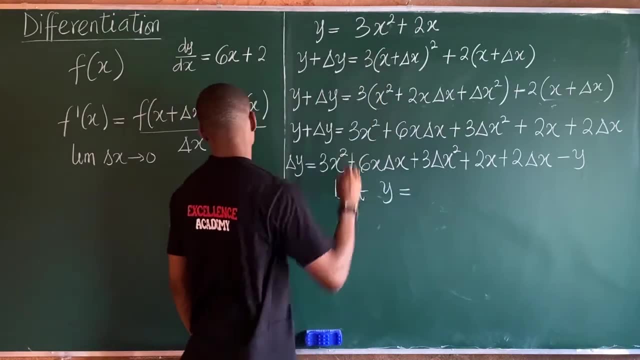 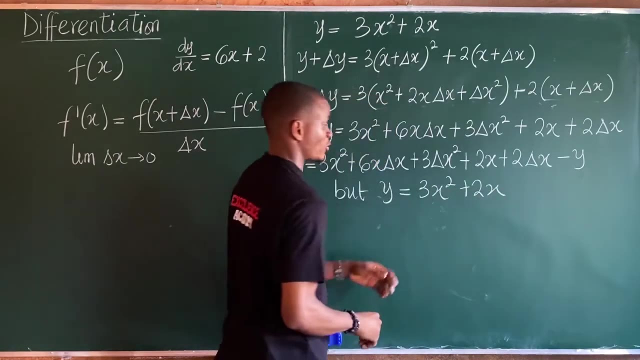 So here's plus y comes here. because what there, Your minus y? All right, But we already have that y is equal to 3x squared 3x squared plus 2x, So I'll substitute this value into this position here. 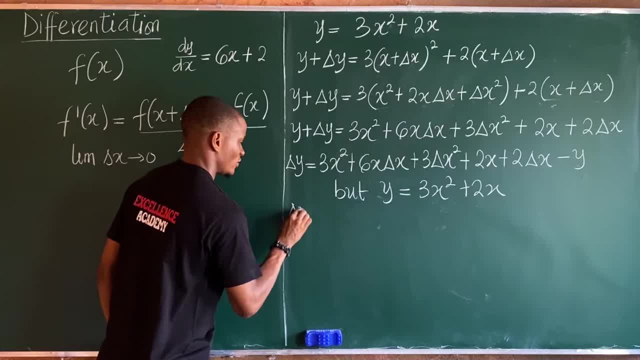 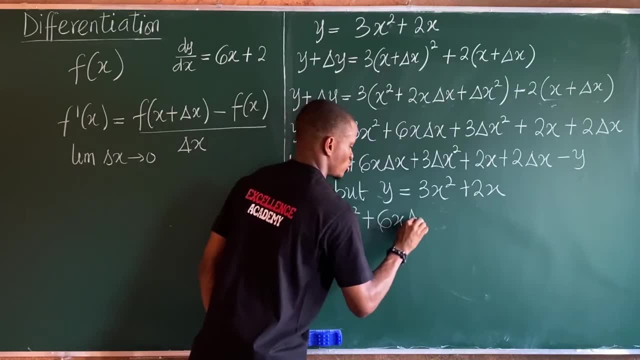 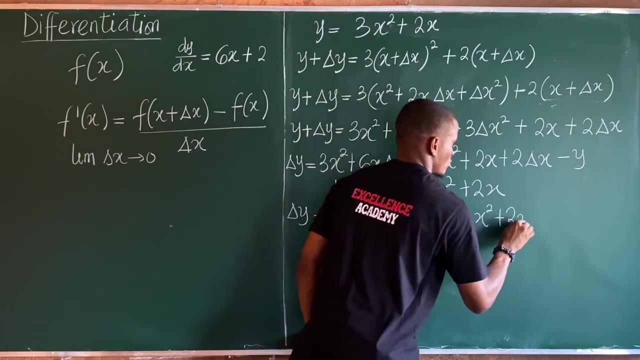 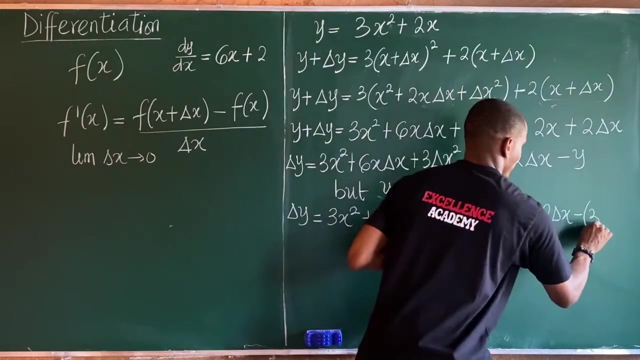 So I'll have that. change in y is equal to 3x squared plus 6x. change in x plus 3. change in x squared plus 2x plus 2. change in x minus y. The value of y here is what 3x squared plus 2x. So this is the value of y here. 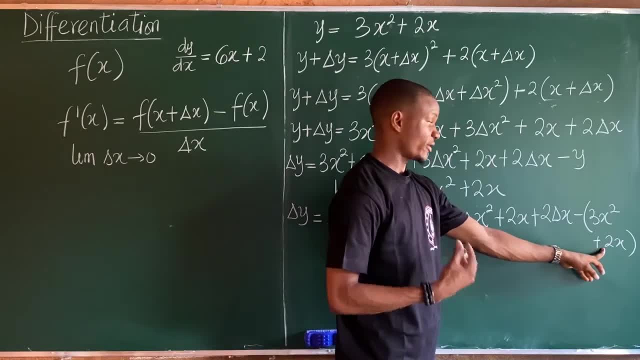 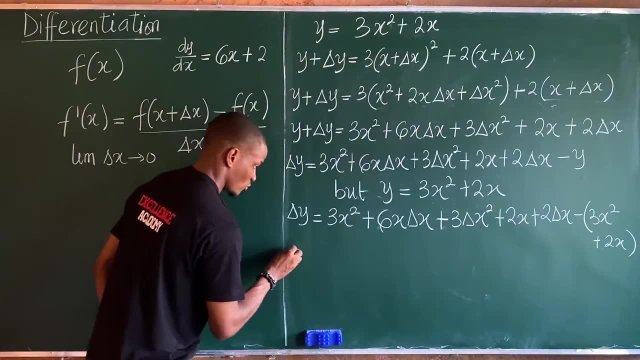 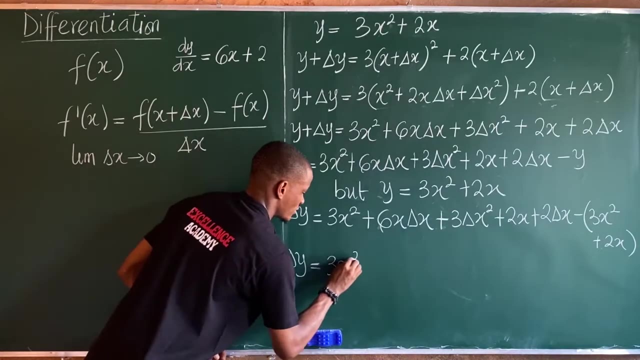 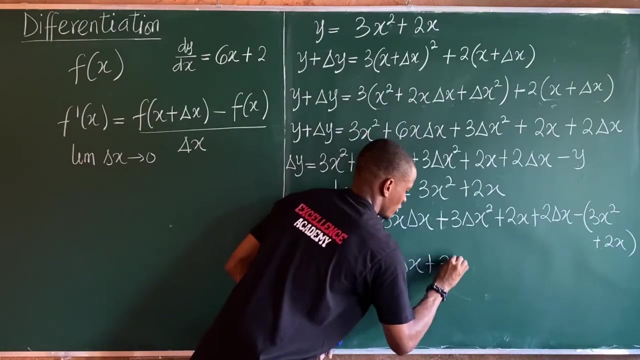 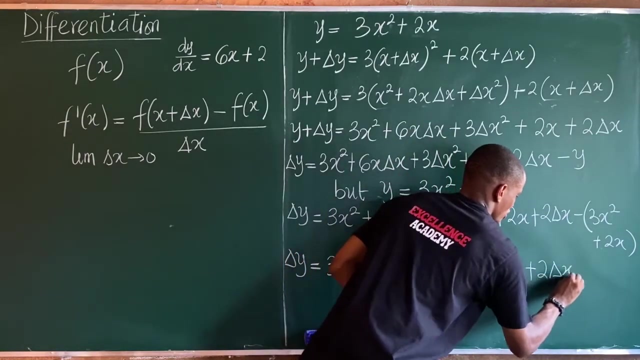 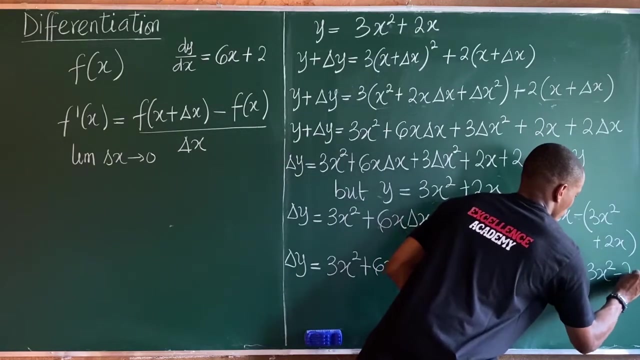 Observe that I encase y in a bracket. Please be very careful with this. So put this value of y here. We'll put it in bracket first. So this is now equal to: I have that. Change in y is now equal to 3x squared plus 6x. change in x plus 3. change in x squared plus 2x plus 2. change in x minus to this minus 3x squared minus 2 plus 2 minus 2x. 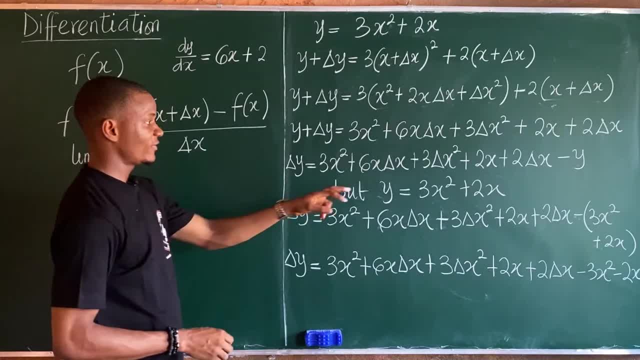 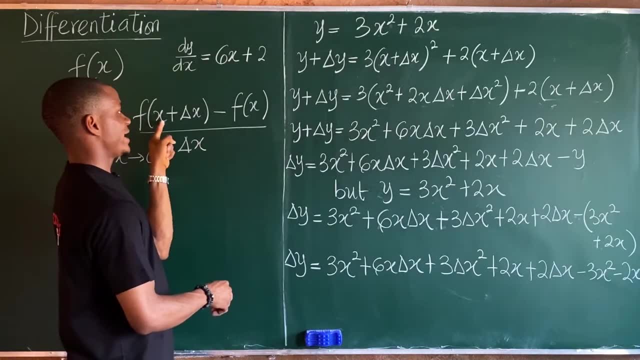 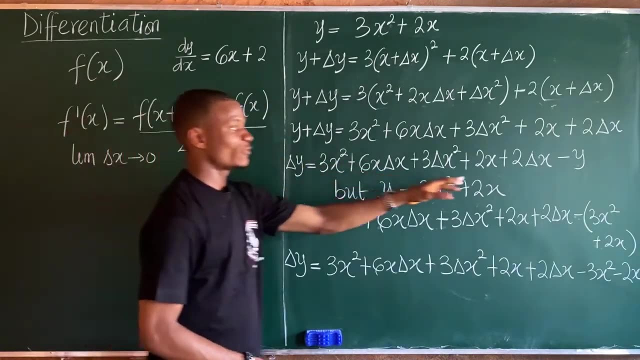 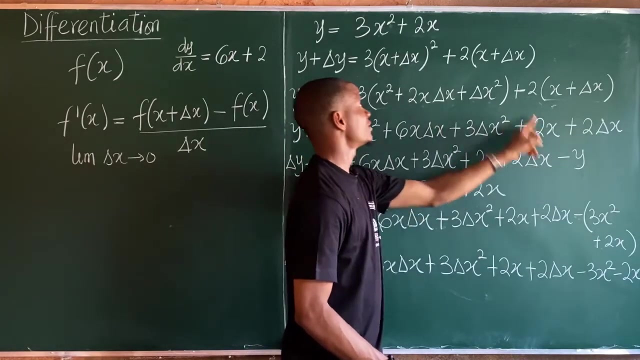 So I have this value. Now notice why I have minus y. here is what you have here. So the first concept is subtract. when you add x to change in x here, subtract this whole value by the function f of x and that's the most. that's what that's what you have here to became. when I added change in x here, this value, I subtracted the main function from this. 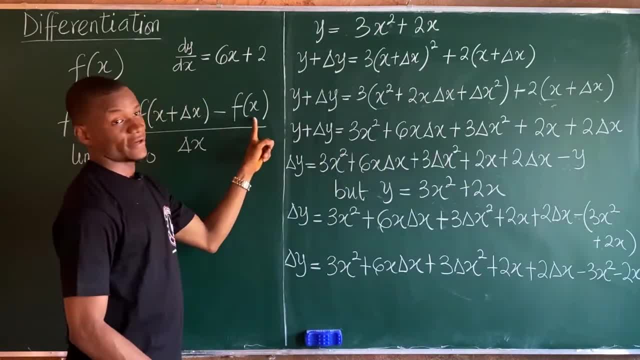 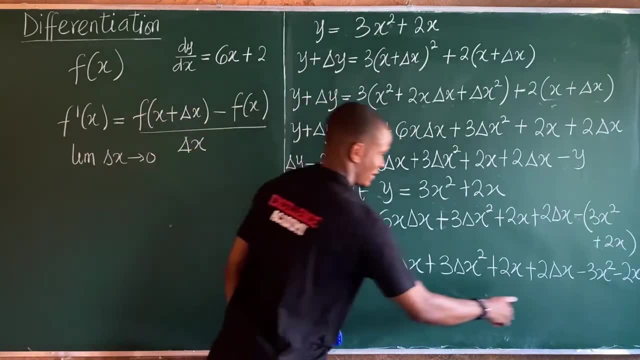 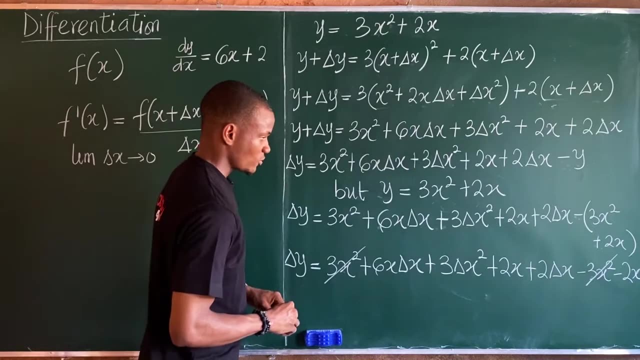 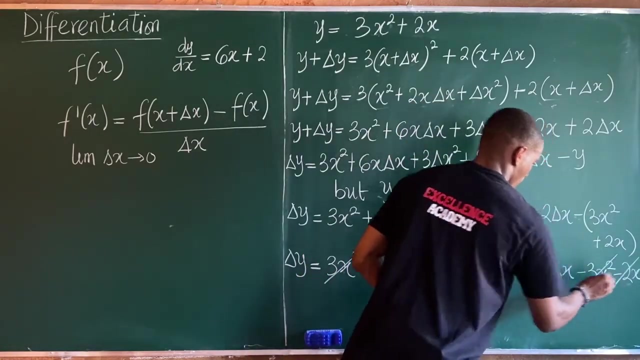 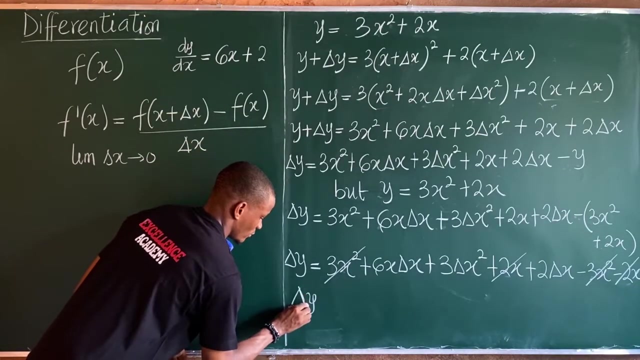 So it became minus y and that's the meaning of what you have here. All right, Now what I have here next up: I can see x squared. I can see minus x squared, so x squared cancels minus x squared. also, I can see 2x. I can see minus 2x, so 2x cancels minus 2x. I'm left with change in y being equal to this is: 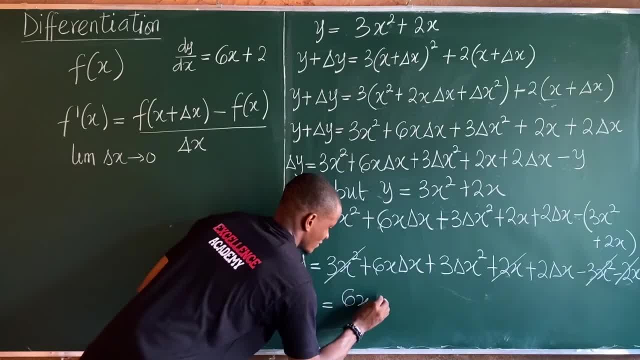 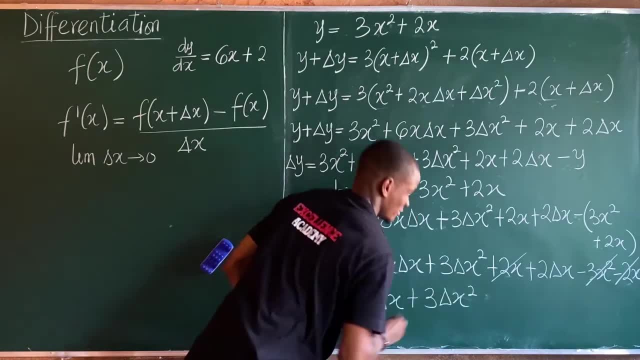 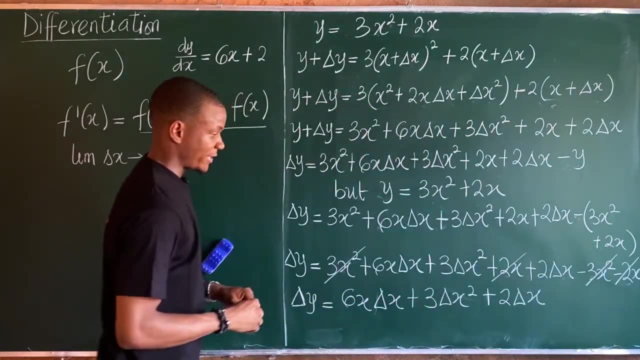 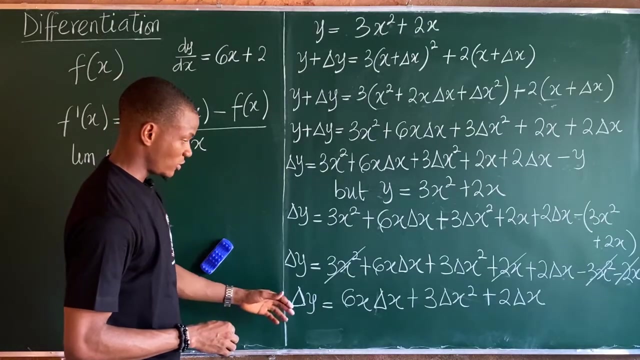 This is 6x change in x and this is 3 change in x. squared, this is plus 2 change in x and I'm having this all right. so at this point here I can see change in x. all of this, that's all through this. next up, I said: whenever you're from this now, next up, I'll divide by. 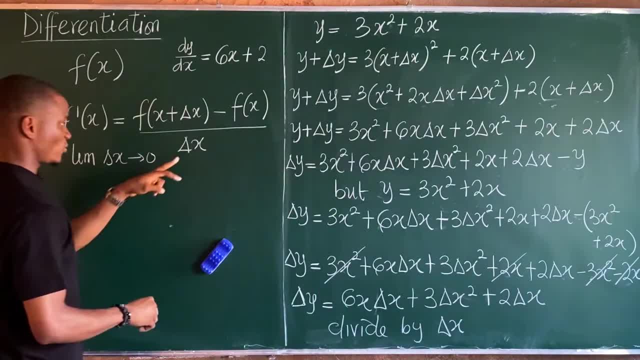 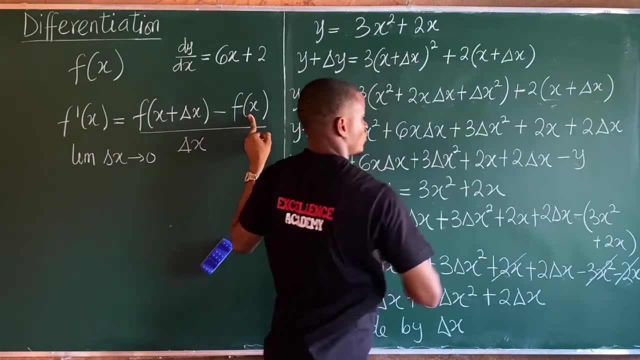 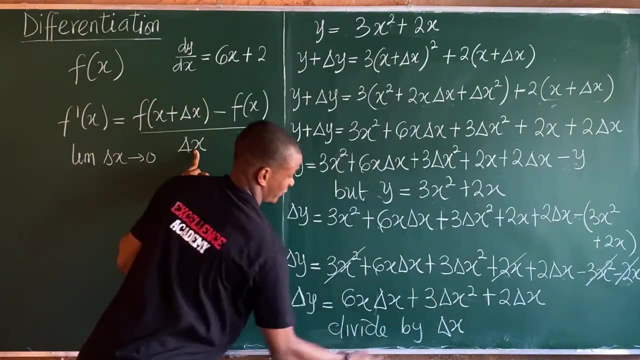 By change in x, and that's what you have this here. this means after subtracting your dysfunction, which is this All right. so, after subtracting and counseling out, collecting like this next up, divide shoe by changing x, and that's what I have here. divide by changing x. this now gives you: 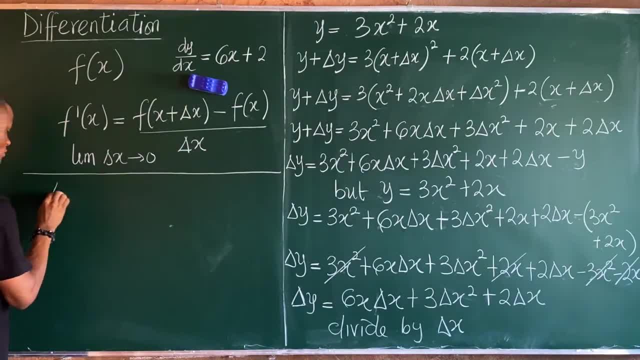 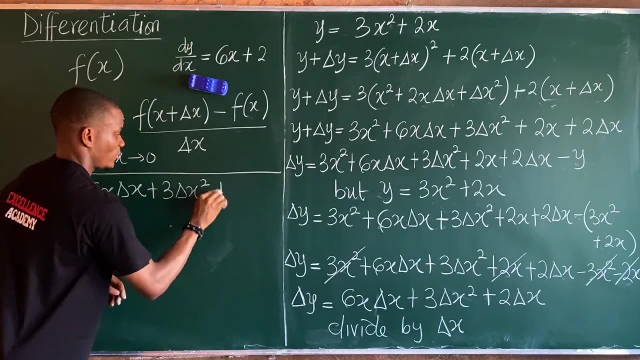 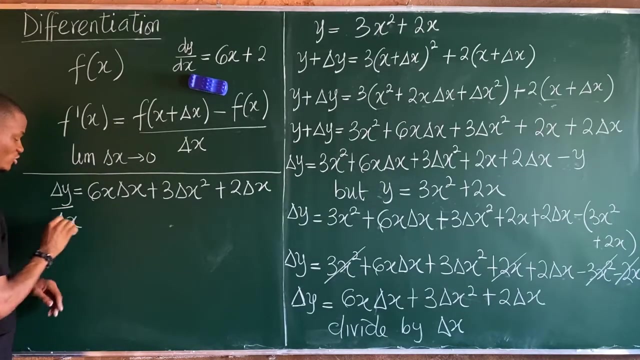 This now gives Change in y As being Equal to 6x. change in x Plus 3. change in x squared Plus 2. change in x we said we are dividing to by changing x becomes here all over. change in x. divide here by what change in x? divide here by what change in x? divide here by change in x.